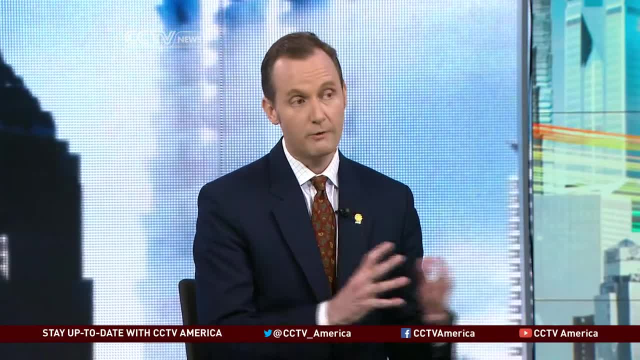 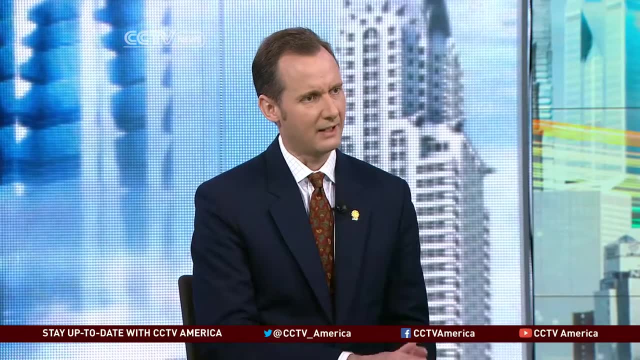 for government is law enforcement, And law enforcement is expensive, especially in a country like Brazil or Indonesia, where you have huge expanses of land and forests are being cleared here, here, here. Where do you send the police this month If you're? 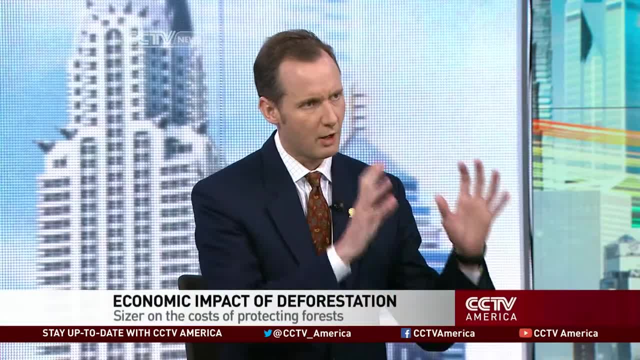 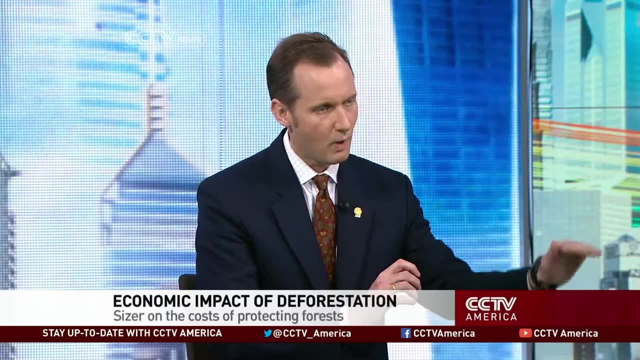 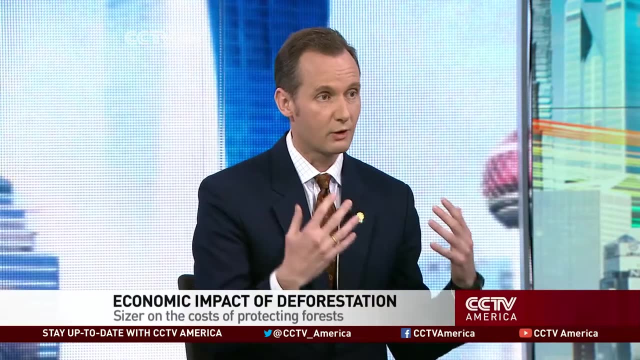 using helicopters. it's very expensive. Global Forest Watch helps them focus those efforts. It shows in near real time where forests are being lost. This month shows you where to go, where to take action, If you're a business leader, a company like Unilever or Nestle using soy beef palm oil. 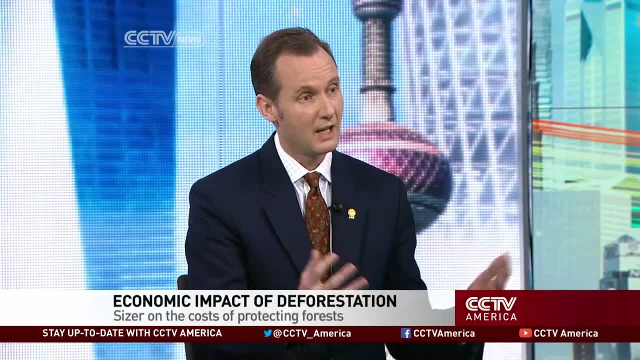 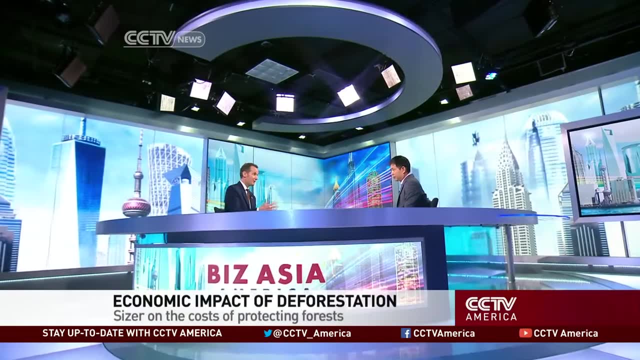 as inputs- agricultural inputs- into your products. you want to be sure that your suppliers are not destroying the rainforest, to put it simply, And they've made commitments to do that. Well, Global Forest Watch helps you keep an eye on those suppliers and see whether they're. 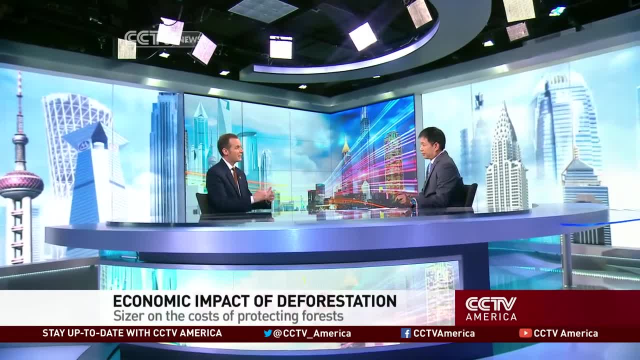 actually doing it, And if you're an NGO or a community leader, you can use Global Forest Watch to help see what others are doing in the forest. NICK SCHIFRIN. Thank you, David. Thank you, DAVID BROOKS. There's been a lot of talk in the press about 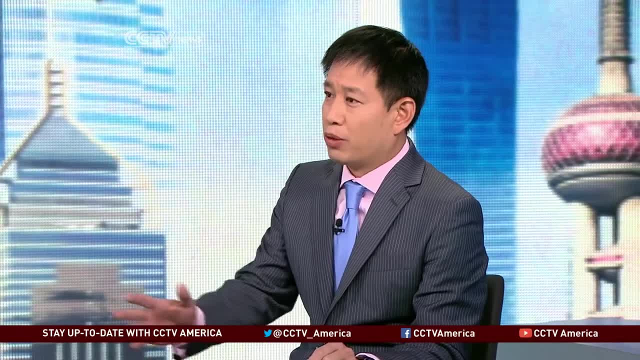 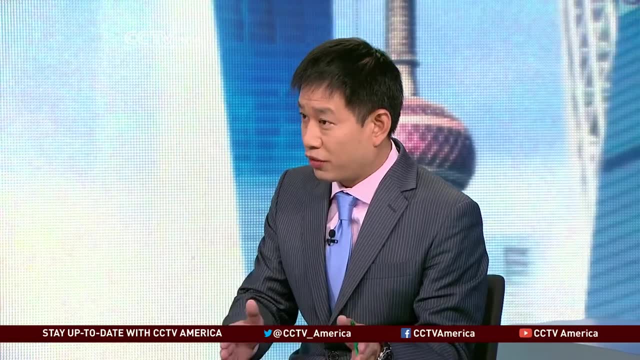 fires, for example, in this case Indonesia, But around the world. these fires are not unique. They happen all the time. The forest, the deforestation, does contribute to a part of that. How does it impact the economy of these governments? Because that's something. 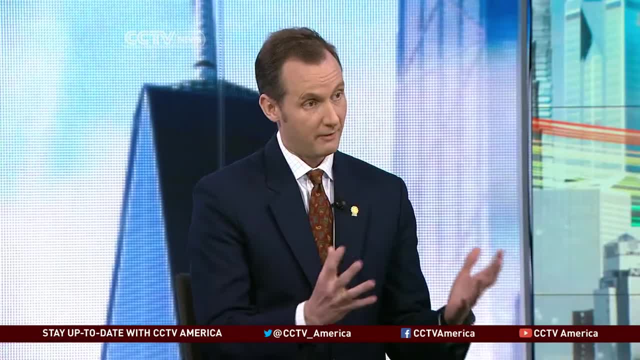 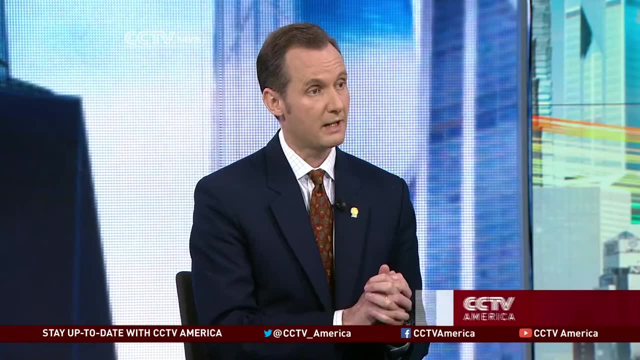 that they're probably thinking about DAVID BROOKS. Well, if you take the case of the forest fires, for example, in Indonesia, Sumatra has had again very serious fires over the last few weeks. The schools have been closed for weeks. 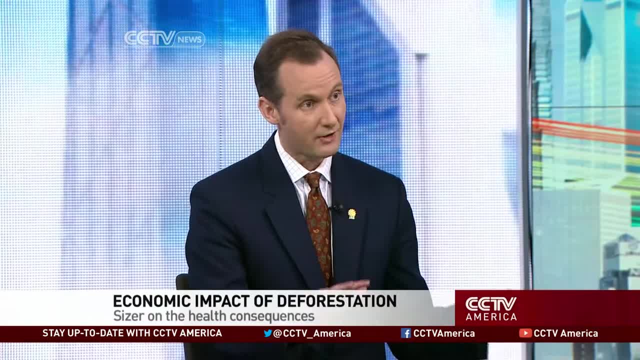 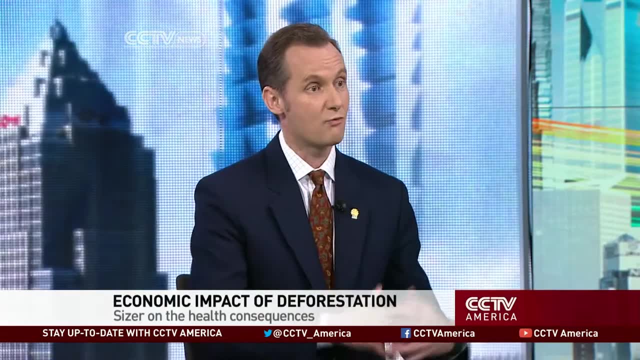 The airports have been closed. It pretty much shuts down the local economy completely. If you look at the fires in California and Australia, you see entire communities having to relocate because of these fires. Again, the economic impacts are phenomenal And the impacts on the health of the people 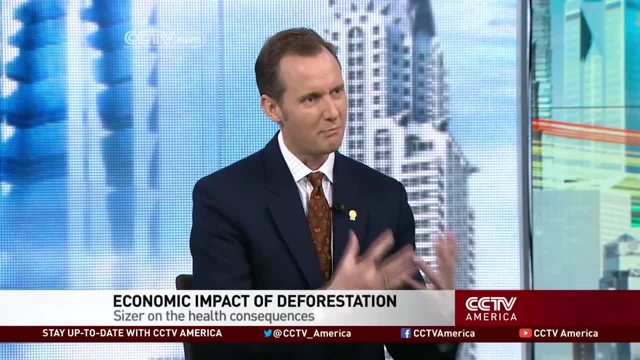 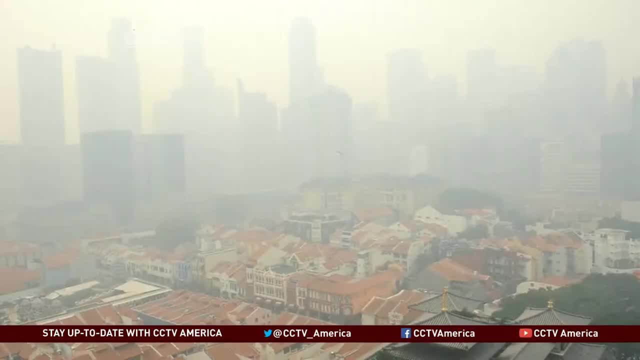 who live in these areas breathing in the smog, the bonfire-like smoke that's billowing across their communities day after day. the impacts are terrific. NICK SCHIFRIN, Is there a specific dollar figure, perhaps, that you can assign to the government or productivity that's lost because of these incidents?